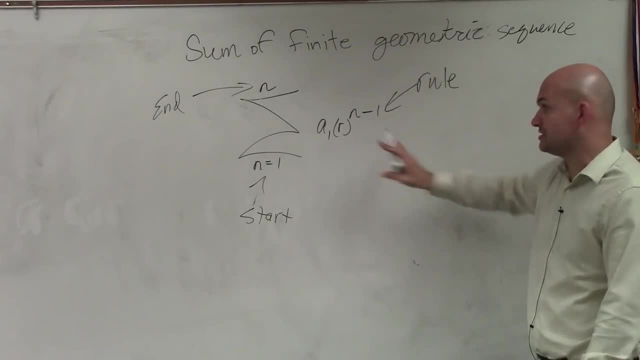 of a finite geometric series when you can have all this information is: s of n equals 1 minus r to the n. I'm sorry, a sub 1 times 1 minus r to the n divided by 1 minus r. All right, So let's go. 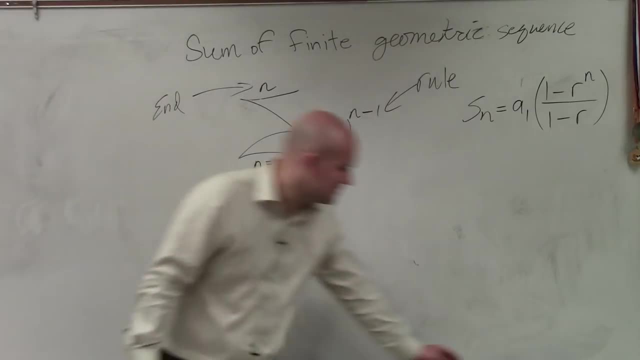 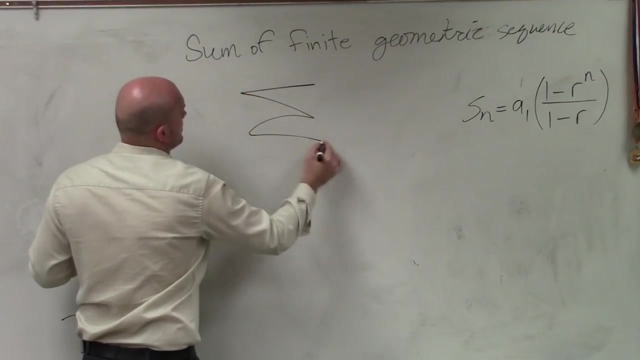 through an example and try to see you know if we can determine the sum. So let's say, I give you a problem and in that problem let's see, let's see this rule I'll do, I'll do a prom off of your. 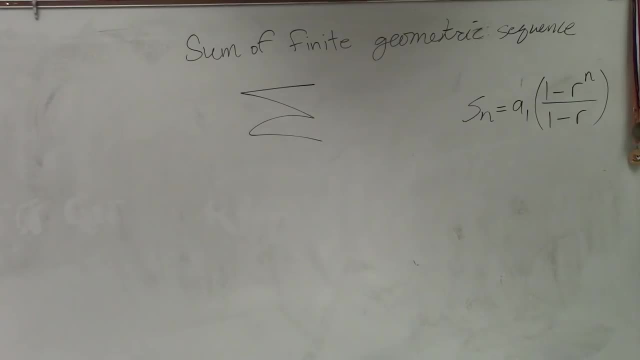 homework: Sigma 6, 1.. One-fourth, One-fourth i minus 1.. All right, So if I was asking you to go ahead, if I was going to ask you to go ahead and find the sum for this, obviously you guys can easily plug 1 in for n. plug 1 in for. 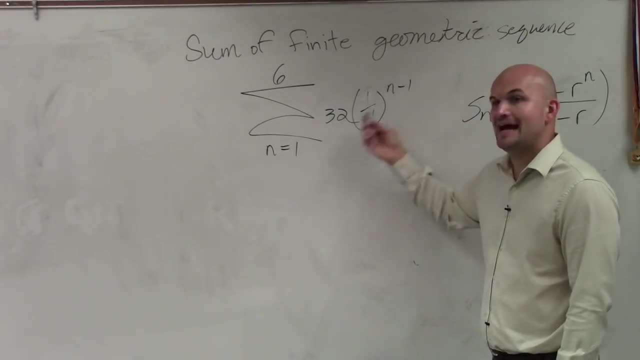 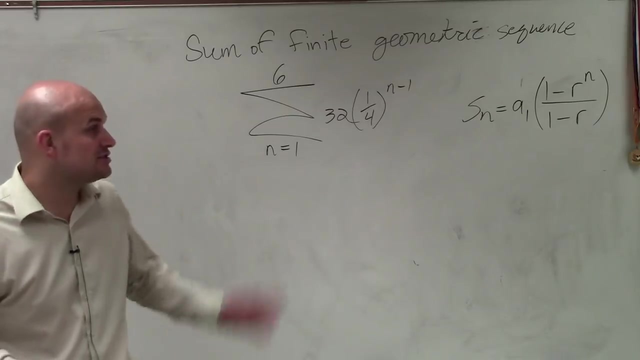 2,, 3,, 4,, 5, 6, add them all up and get the answer right. But it also would be helpful to just go ahead and plug all the information into the formula and then you only have to do the math. 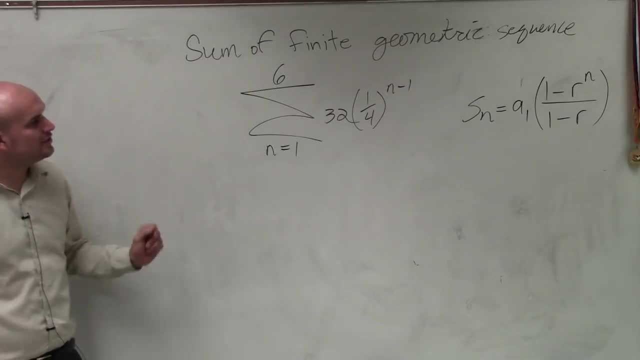 once and you can combine everything right. So what we're going to do here is we need to be able to identify. do we have the terms of the formula Now? remember the rule is in the format: a sub n equals a sub 1 times r to the n minus 1.. So a sub 1 is what we're multiplying by our rate, So you. 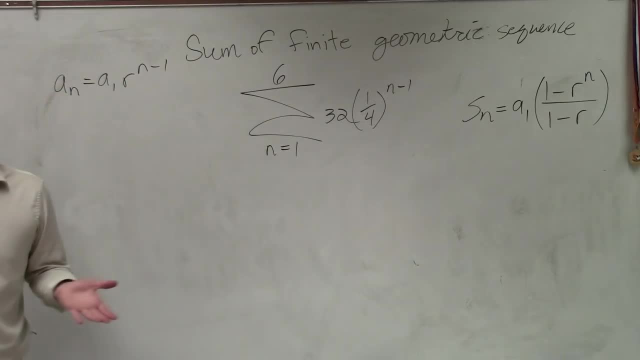 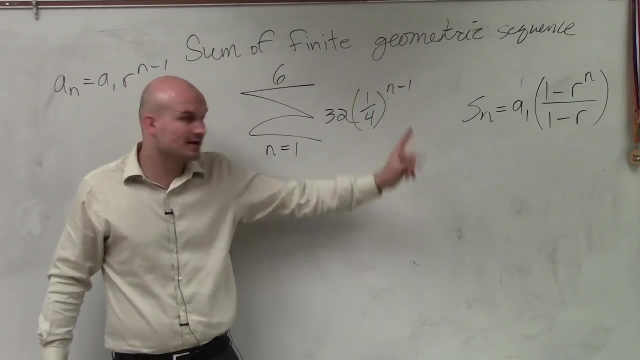 guys can say that a sub 1 is 32.. If you want to check that, just plug in 1 in for n. 1 minus 1 is 0.. 1 fourth raised to the 0 power is 1.. 1 times 32 is 32.. So you guys can see that the first term 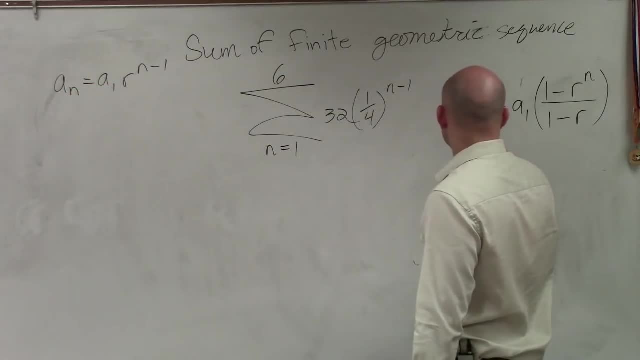 would be 32 anyways. So let's go ahead and plug this in. So I have s of n equals 32 times 1.. Let's get a little more space. s of n equals 32 times 1 minus 1. fourth, raised to the 6th, over 1. 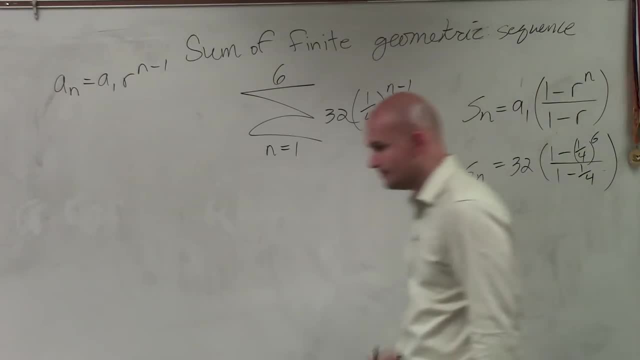 minus 1 fourth. right Now, just a quick reminder: 1 fourth raised to the 6th equals 1 to the 6th over 4 to the 6th. OK, So obviously 1 to the 6th is just 1.. So we do need to compute 4 to the 6th power. 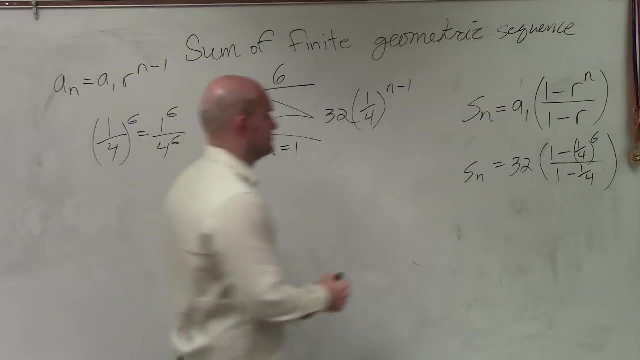 which is 4,096.. So I have s of n and then 1 minus 1 fourth is 3 fourths. So I have 32 times 1 minus 1 over 4,000.. So I have 4,096 divided by 3 fourths. Now obviously I can rewrite. I'm going to do a little math over here. 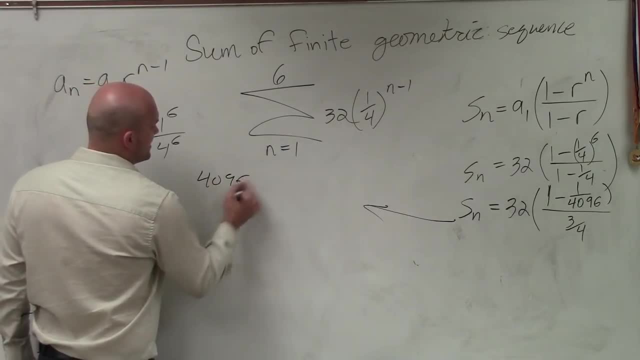 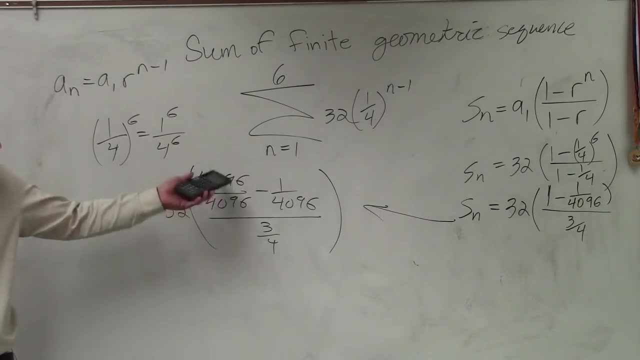 Obviously, I can rewrite 1 as 4,096 over 4,096 minus 1 over 4,096 divided by 3, fourths times 32.. Does everybody follow me with my fractions? No, What did you miss? Yeah, that's 1, right, So I just rewrote that. 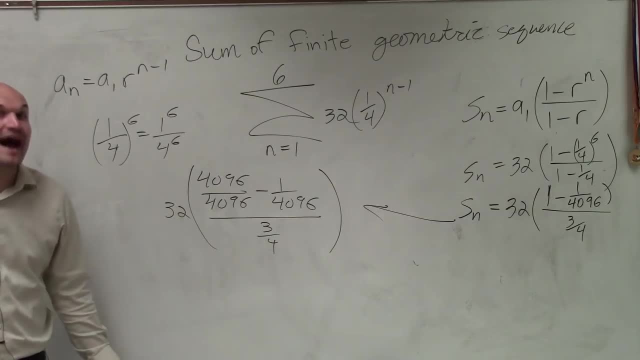 So obviously you can see that this answer is 4,095, right minus over 4,096.. And this is all times 32.. So I can say 4,095 over 4,096 divided by 3, fourths times 32.. 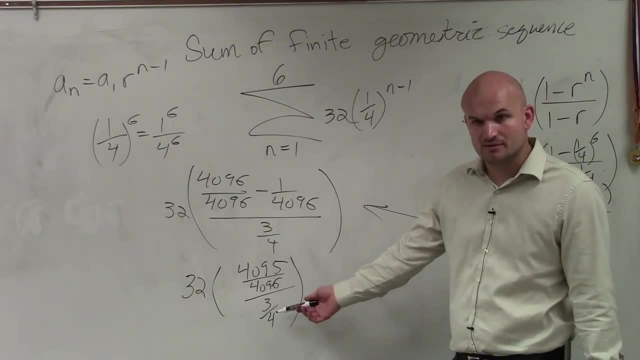 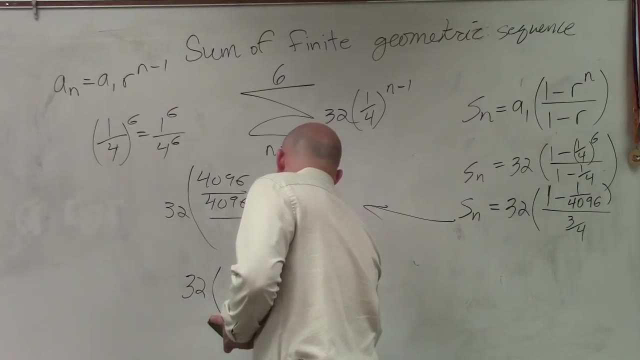 Now one thing we can do is we can simplify this fraction, right? Yes, So rather than dividing by 3 fourths, I can multiply by the reciprocal times 4 over 3 on the top and the bottom, And when doing that, that takes that to 1.. 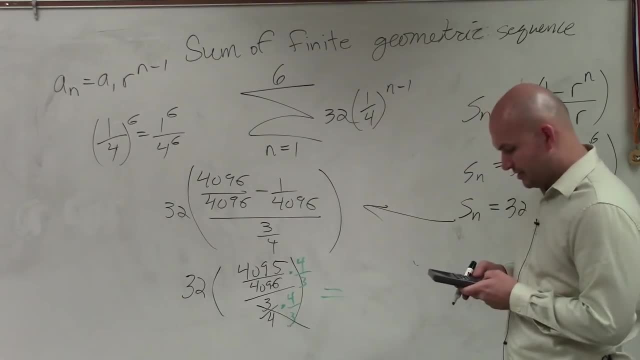 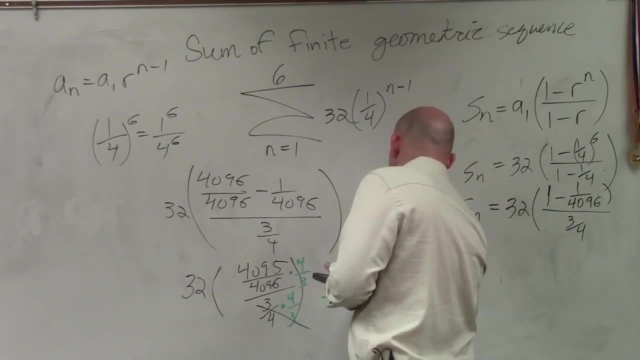 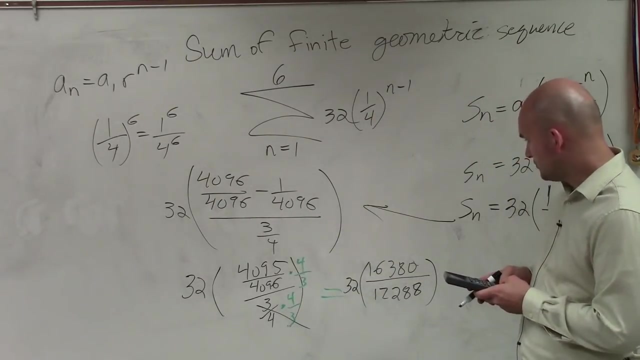 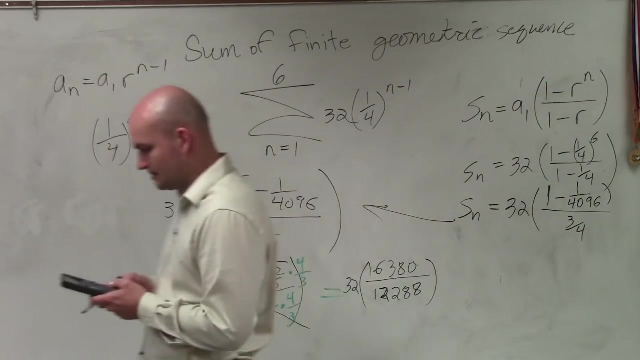 So now I'm left with 4,095 times 4 equals 16,380 divided by 4,096 times 3.. 3 equals 1,288 times 32.. Multiply 32 times 16,380.. Divide that by 1,288 and then reduce my fraction.